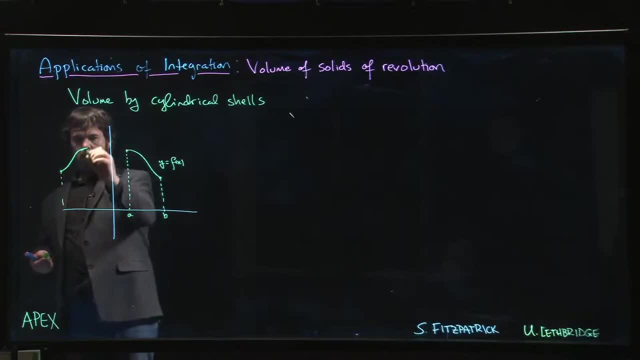 we're going to revolve this around and we're going to generate this solid like so, all right, like so, Okay. so we can kind of see the region that's generated here right when we revolve this thing around, And of course, the middle is cut out. so we're going to revolve it around the 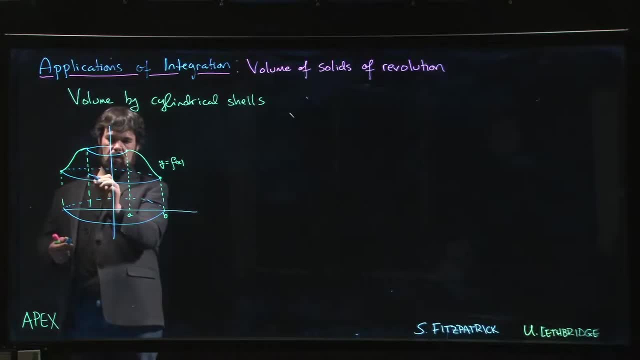 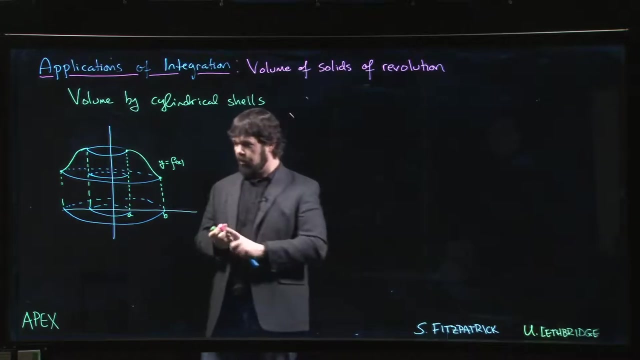 middle. so we want to account for that too at each of these. All right, so we're cutting out this middle bit. Okay, so there's the solid that we're interested in Now. we could, of course we could- do this using washers. We know how to do this using washers. We could try to draw the. 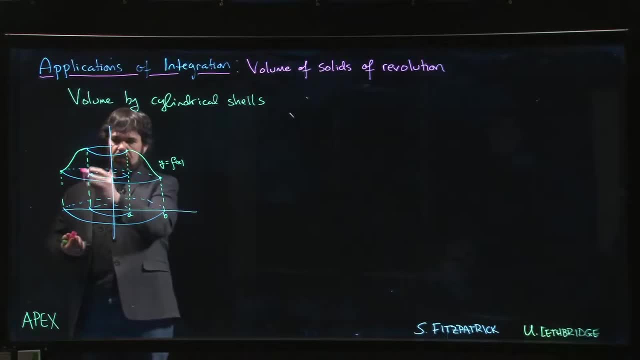 washer in here at a given height. but one of the things you'll notice is that the washers that we use they're going to change halfway down because we move from working along the curve to working along the vertical curve. So we're going to do this using washers. We're going to do this using 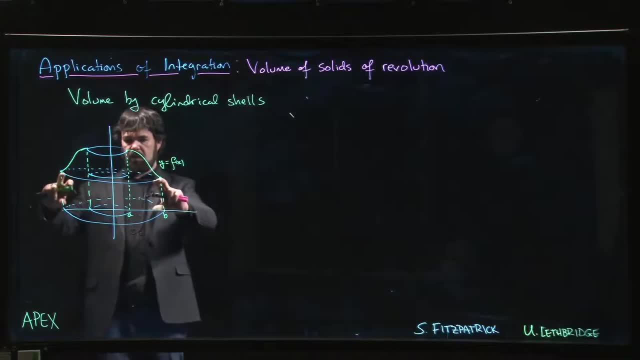 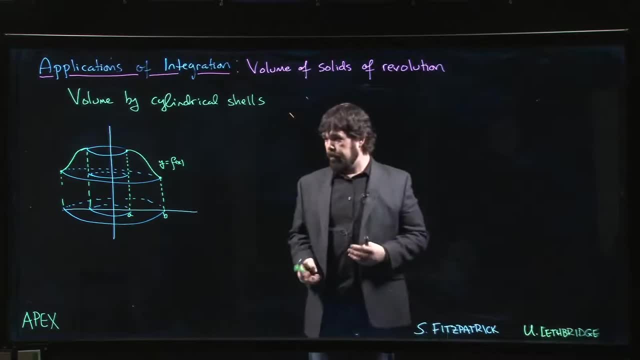 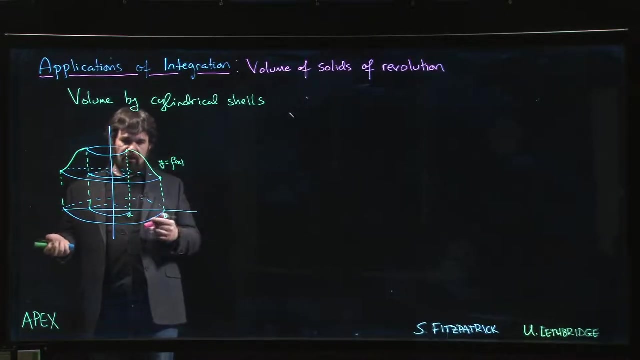 both of them, and that's relatively straightforward. right? It's just going to be volume of a cylinder, right? Volume of the big cylinder minus volume of the small cylinder. That's a simple calculation. You don't even need calculus for it. Okay, so we could do it in kind of two pieces and patch them. 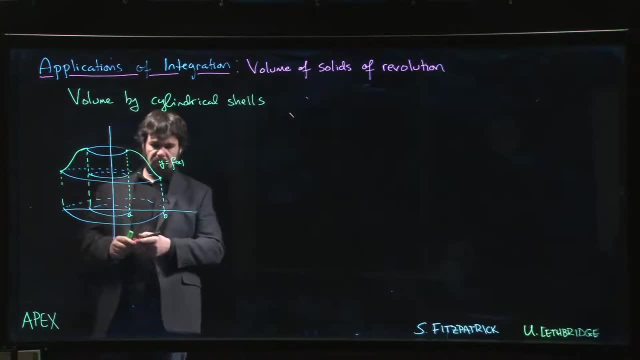 together. but it turns out there is another method that you can use. You can use what's called a cylindrical shell method. So the idea here is, rather than doing washers and integrating with respect to y, we're going to do shells and integrate with respect to x. So the way it looks, 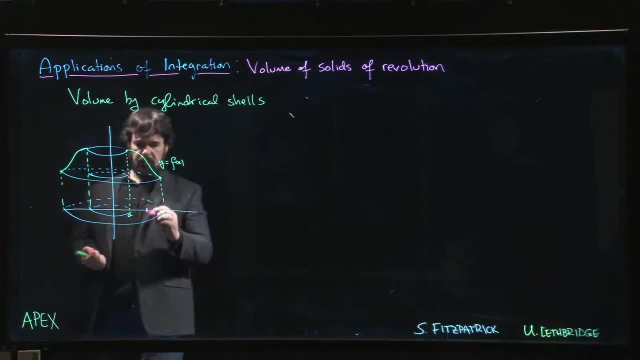 is like this: We choose a particular x value, We travel up until we hit the curve, down from the curve, okay, And we imagine just taking this vertical line segment and revolving it about the axis. So if we take that vertical line segment and revolve it about the axis, we're going to do: 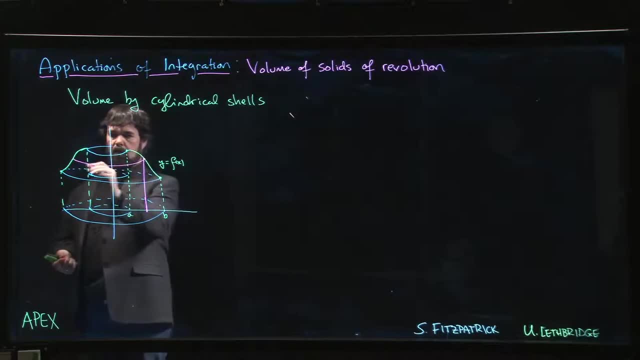 that vertical segment and we revolve it about the axis. okay, We generate a cylinder. right There's a cylinder And remember that the area for that- you know the surface area of that cylinder, because we're not including the top or the bottom right- What is the surface area of? 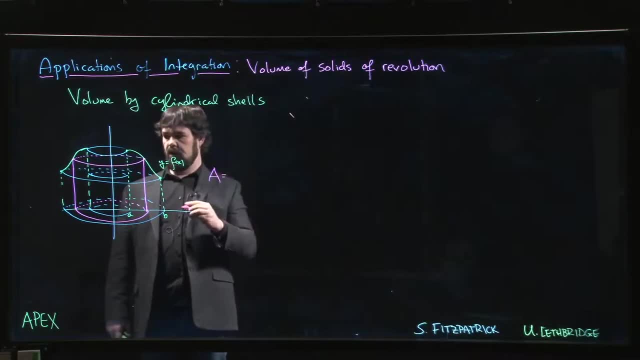 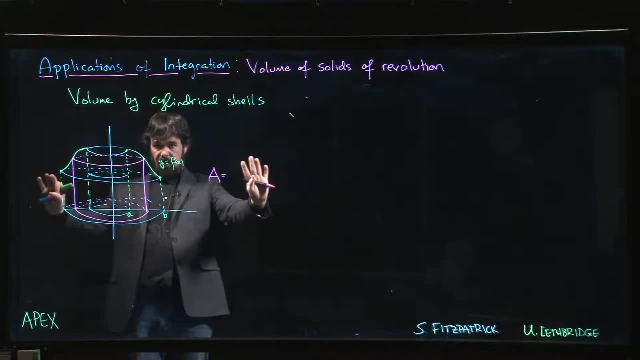 area of that cylinder is the area of the cylinder. So we're going to do that. So the area of that cylinder is, if you, you know, imagine cutting it. If you cut that cylinder and lay it flat, you get a rectangle right. The height of the rectangle is, or the height of the cylinder is the height of. 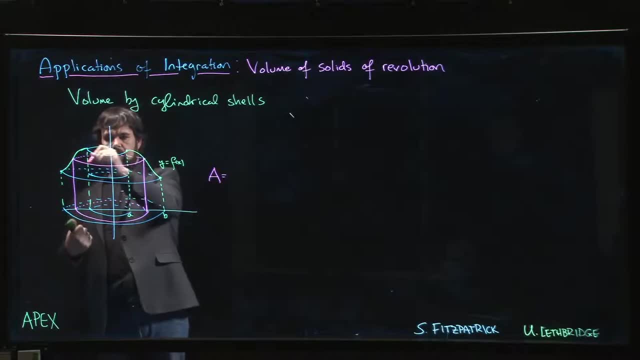 the rectangle. The width of the rectangle is the circumference of the cylinder, right. So the area is 2 pi r times h. okay, That's the surface area of that cylinder that we've drawn in. okay, Now that area actually depends on x. okay, The radius is just x, right? The radius of the cylinder is: 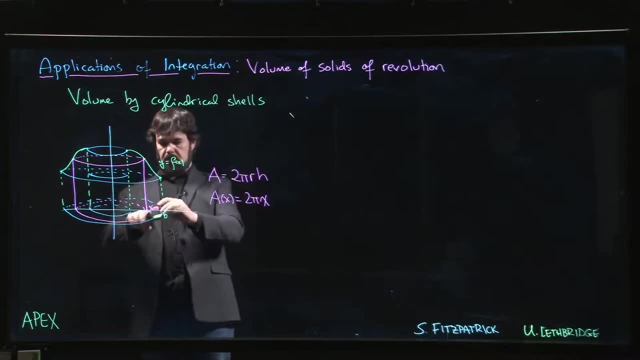 just x, x, The height of the cylinder. well, that's f of x. all right, It's just the y value, okay, So we can express the area of the cylinder in terms of x, And then you can imagine that you. 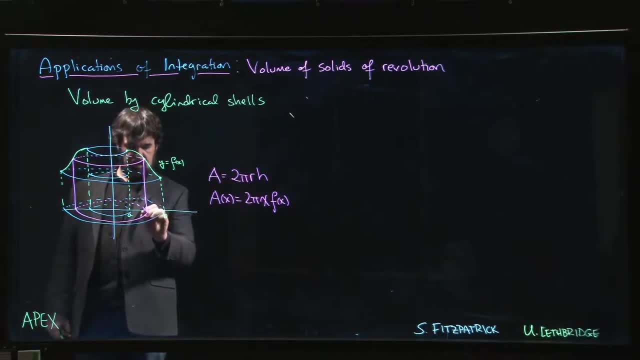 might thicken that cylinder slightly. So you, you know, you thicken it by like an amount delta x, right? So you imagine it's like a tin can, right? So if you thicken it up, you add some tiny sort of. 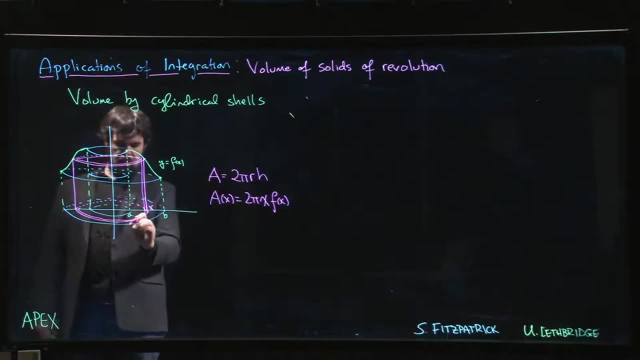 infinitesimal thickness to your cylinder. well then, it occupies a certain volume of metal, right? If you take a tin, can you know? cut the top and bottom off, you lay it flat, get the area, calculate the thickness, you can figure out how much. you know what the volume of metal in your 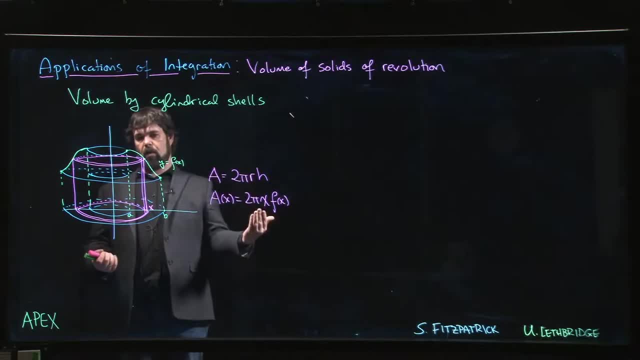 can is okay. So what you can do is for each x value, starting at a and ending at b, you get one of these cylinders. Area: surface area of the cylinder is given by that. Thickening by an amount dx gives you an infinitesimal.